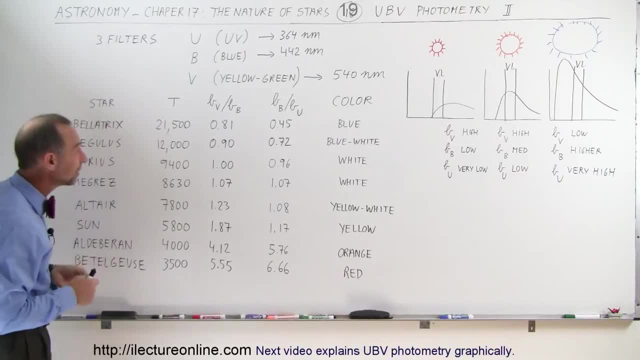 which has a surface temperature of 21,500 degrees Kelvin- Pretty hot. Notice the ratio BV to BB, meaning it's less than one. You can see that the energy of the blue light range is much stronger than the energy of the rest of the visible light spectrum. 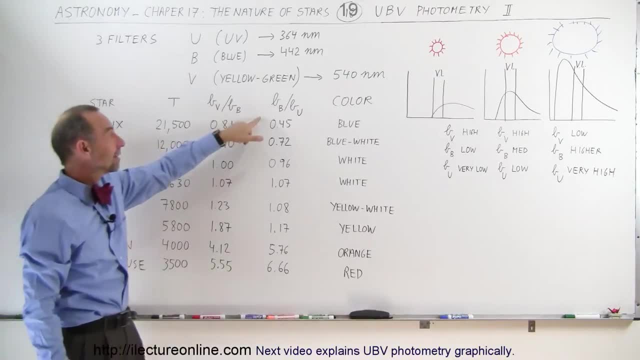 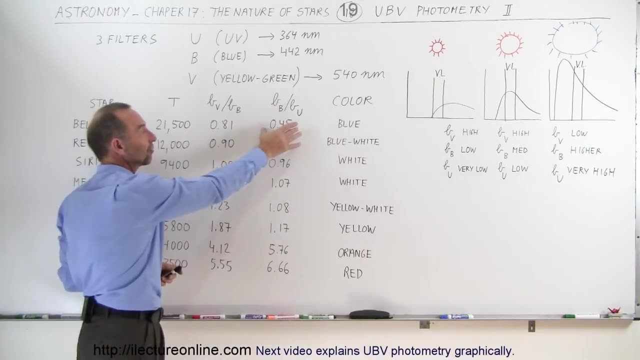 So therefore we have a ratio less than one, And then we can see that the energy coming through at the UV spectrum is much greater than the energy coming through at the blue light spectrum. So the ratio there is far less than one. 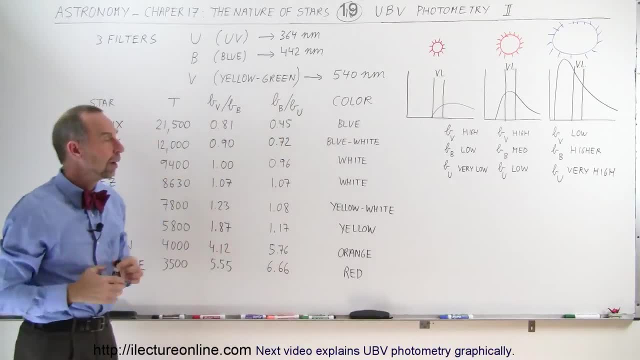 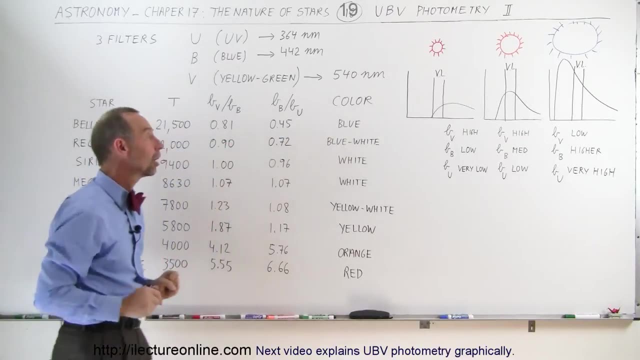 This would indicate a very hot star, probably with a very dark blue color. Well, I shouldn't say dark blue, because they don't have that dark blue color, but definitely a strong one. They have a strong blue color associated with that type of star. 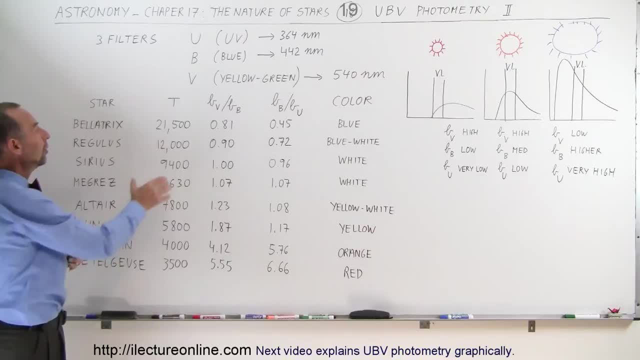 The next star, Regulus, which is the brightest star in the constellation Leo, with a surface temperature of 12,000,, has a ratio of the visible light spectrum to the blue light spectrum of 0.9.. That's a little higher than 0.81.. 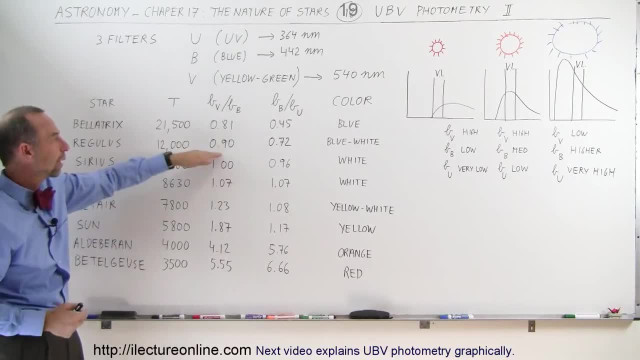 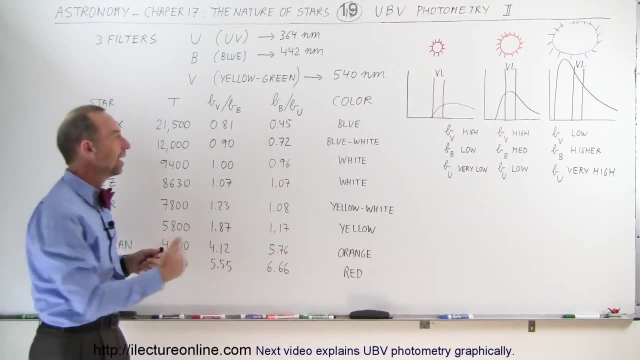 So that means a little bit more of the visible light is coming through relative to the blue light And you can see that the ratio of the blue light to the UV is not as small you could say. In other words, the UV radiation is not as predominant. 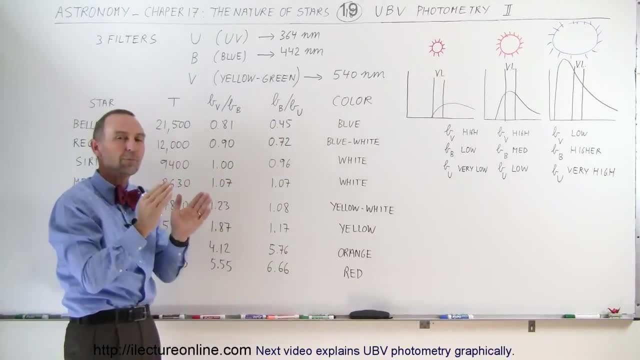 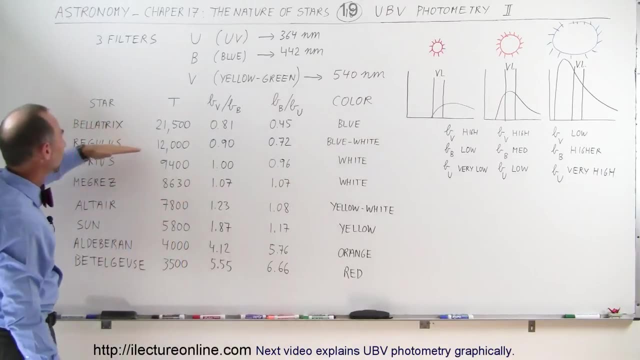 compared to the blue radiation, which you can then see, that it shifts a little bit more from the blue towards the visible light spectrum and therefore associated with a blue-white color and therefore associated with a lower surface temperature. The next star, Sirius, the brightest star in the sky. 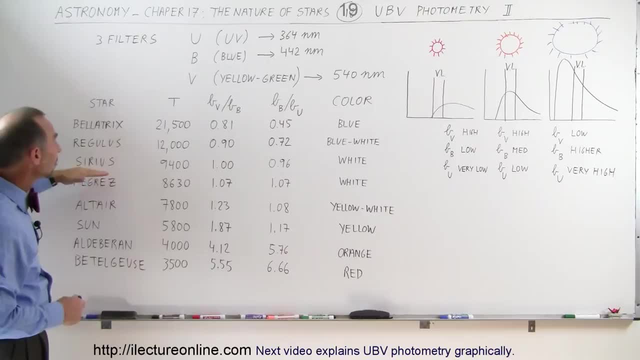 also the brightest star of the constellation Canis. Major surface temperature of 9,400.. Notice that the ratio of the visible light to the blue light is 1 to 1, and the ratio of the blue light to the UV is almost the same. 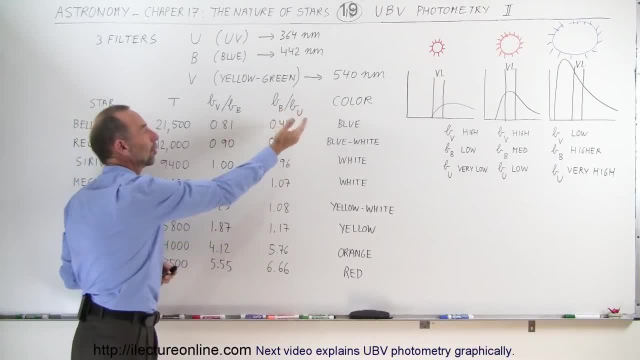 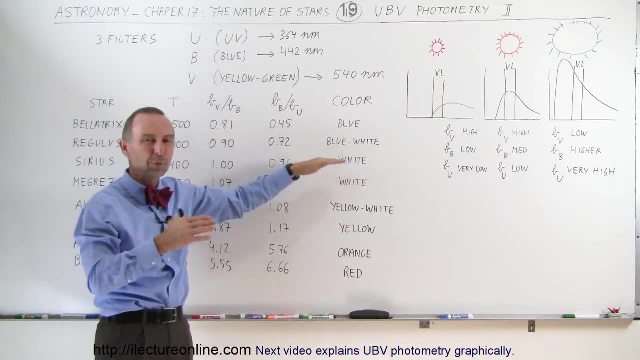 That's 1 to 1 as well, meaning a slightly higher UV band or UV radiation energy than blue energy, and that then indicates that it's the widest looking star, kind of like white, white-blue, But again, Sirius, when you look at it it's a very bright star and has its widest color to it. 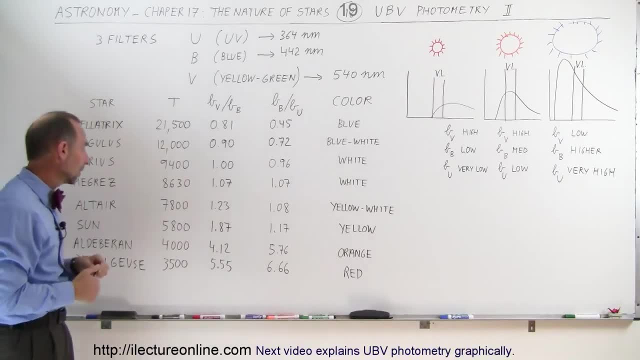 Magris, which is one of the stars in the constellation Ursa Major, or the Big Bear, you can see a surface temperature of 8630,- excuse me- with a ratio of visible light to blue light now greater than 1, meaning it is now more shifted towards the visible light. 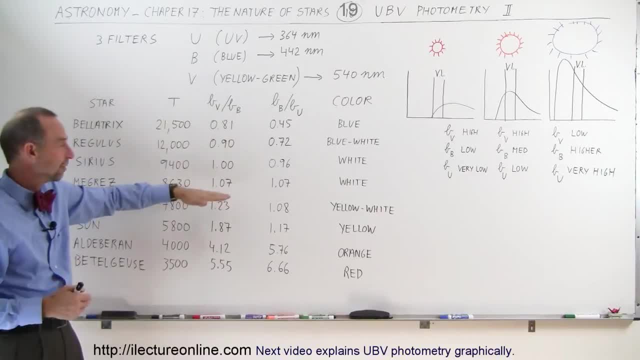 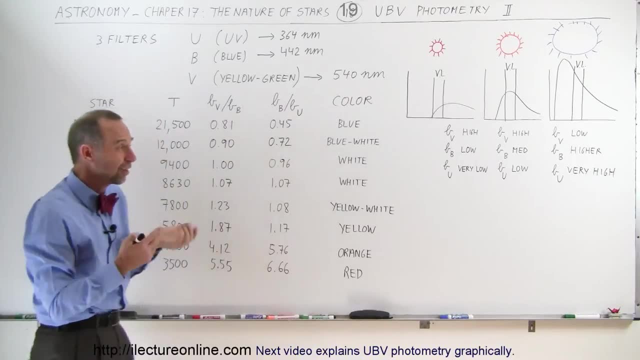 Visible light is becoming a lot stronger and has more energy at the visible light spectrum than at the blue light spectrum. And notice that it has more energy at the blue light spectrum compared to the UV spectrum. So therefore it's shifting away from having the predominant energy in the UV. 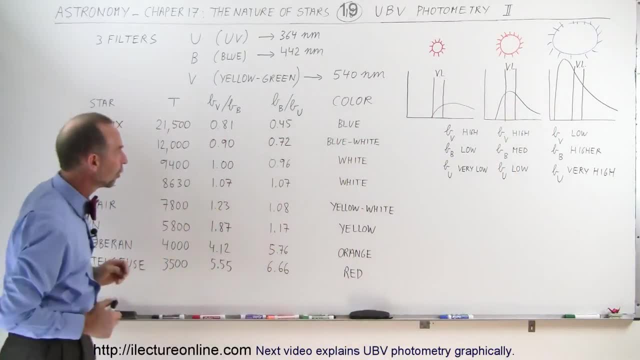 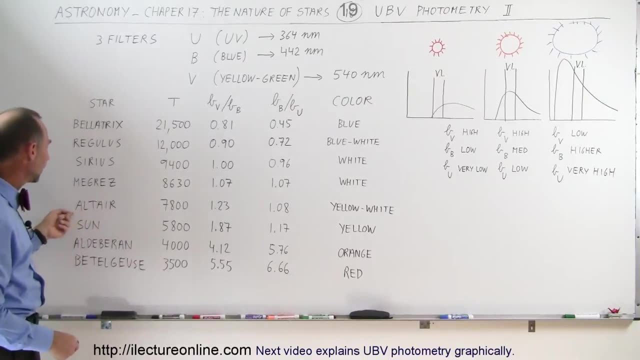 to the predominant energy in the visible light, So you can see that it's beginning to shift over. and then the color of Magris is also the widest looking star, still pretty hot. Then the next star, Altair, which is a star in the water bearer. 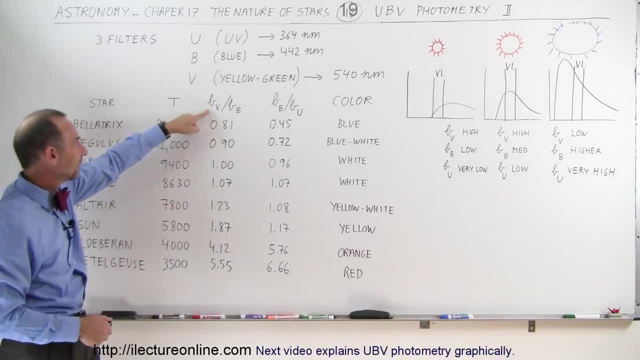 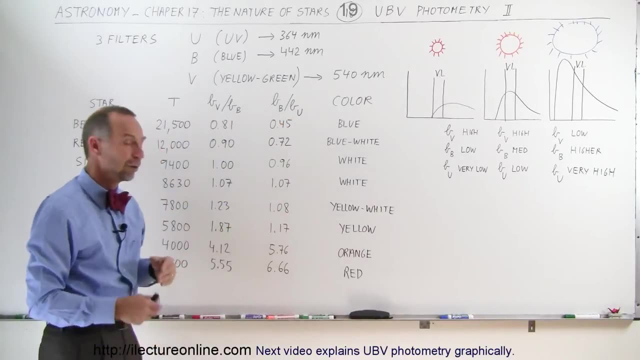 which is at 7800 surface temperature. Notice that the visible light spectrum is now quite a bit stronger than the blue light spectrum, and the blue light spectrum is stronger than the UV light spectrum, So again that shifts it more into the visible light spectrum. 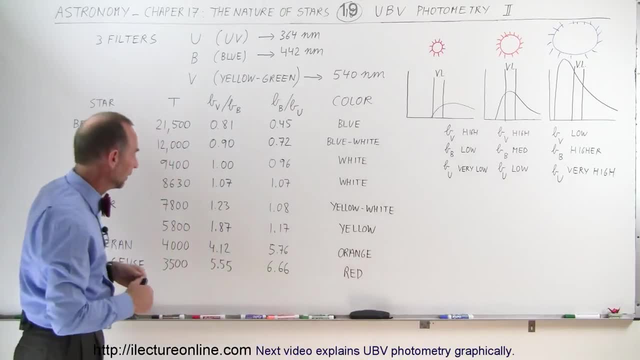 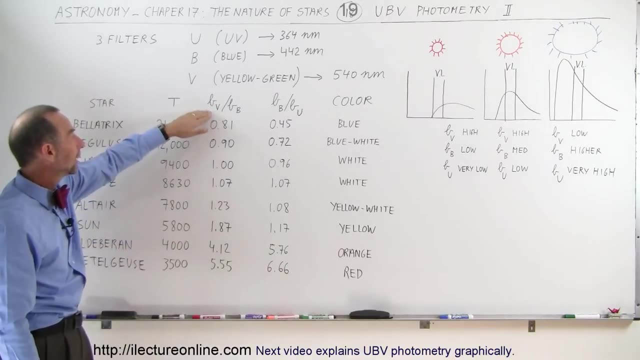 and from white now it's going to the yellow-white color. Then we go to our Sun. We know where our Sun is. surface temperature: 5800 degree Kelvin. Notice how much more we get energy through at the visible light spectrum compared to the blue light spectrum and how much more of the blue compared to the UV. 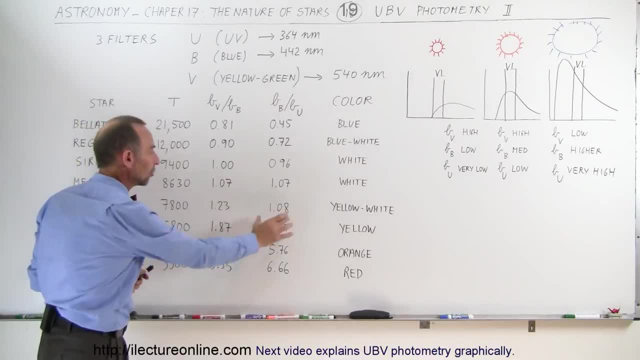 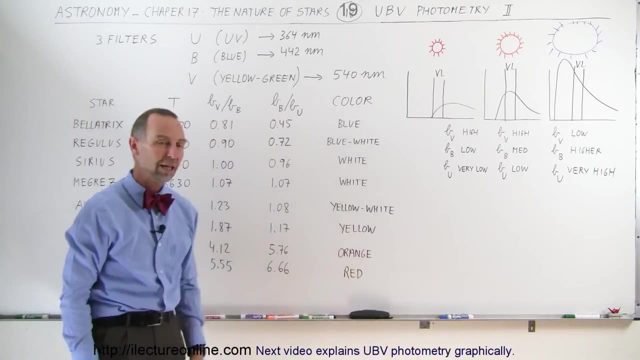 which then indicates: since this ratio is much greater, this one doesn't change as much, but this ratio is much greater. we know that it shifts more into the visible light spectrum and therefore it's associated with the yellow star, like our Sun. 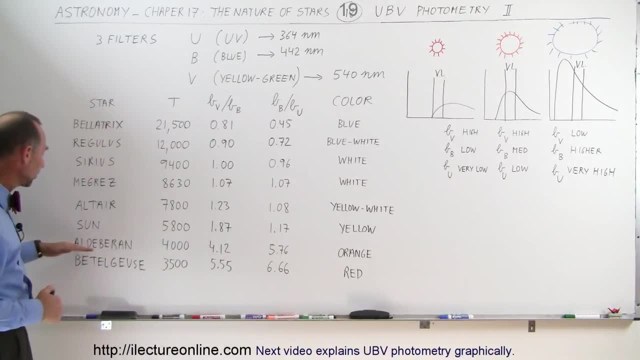 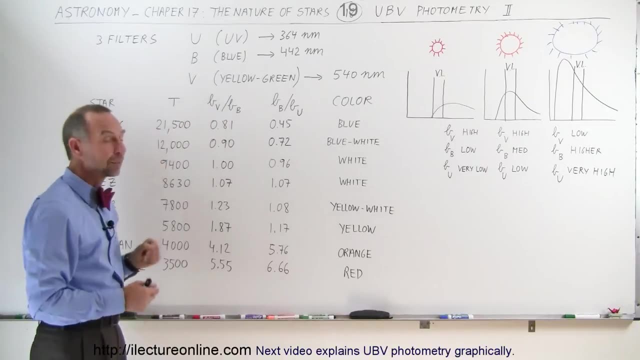 So next star here is Aldebaran, which is the bright star in the constellation Taurus, 4000 degree surface temperature. Notice a large ratio of visible light brightness to blue light brightness, which means it really has shifted over into the visible light. 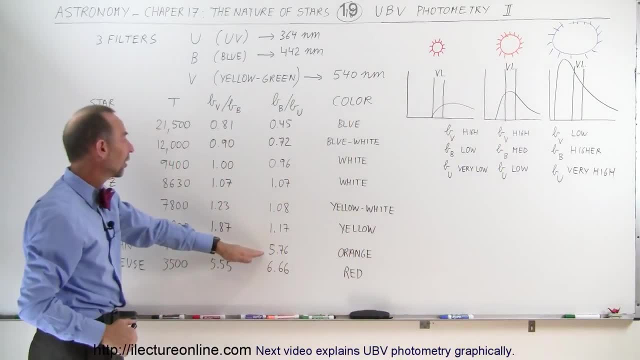 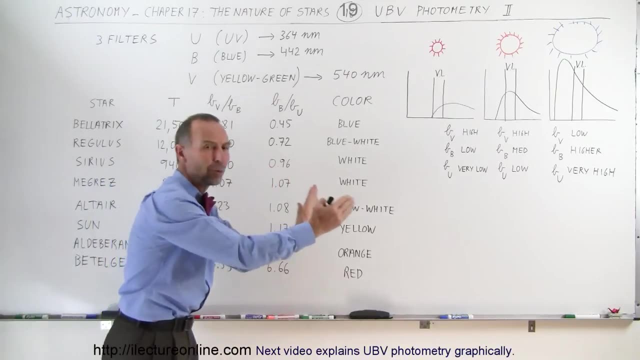 away from the UV and the blue light And notice a very large ratio again from the blue to the UV, meaning very little UV coming through, which we know caused it to shift quite a bit to the right of the spectrum, quite a bit to the reddish-orange color. 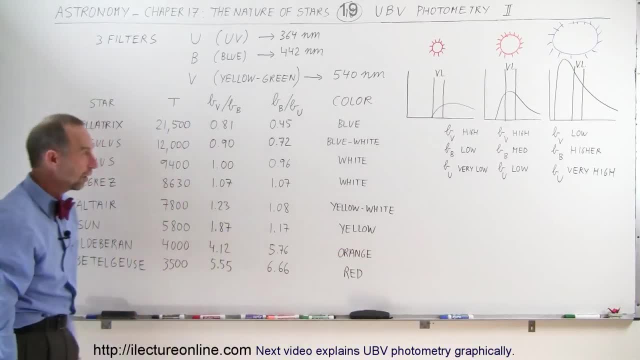 and so, therefore, that star is indeed an orange-looking star. And finally, Betelgeuse, that very large star in the constellation Orion, surface temperature 3500, we know this is a big red giant. Notice the ratios for visible to blue and blue to UV.